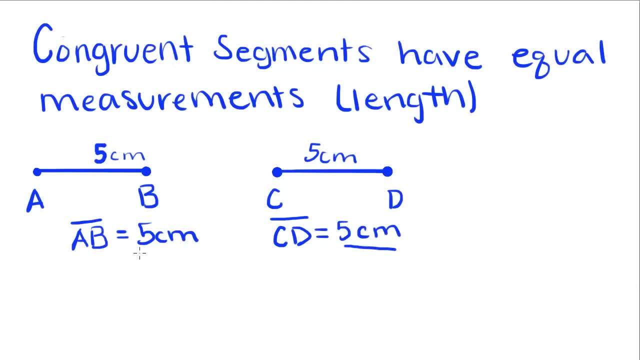 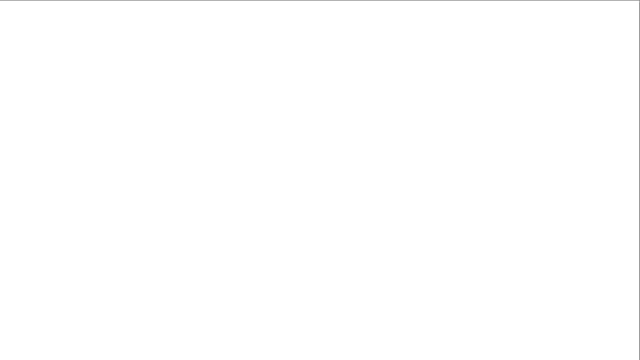 And since they have equal length, we can say that line segment AB is equal to line segment CD, Or that AB and CD are congruent line segments. Okay, alright, Let's say you're given this information, Okay, And they want you to find the length of line segment AD. 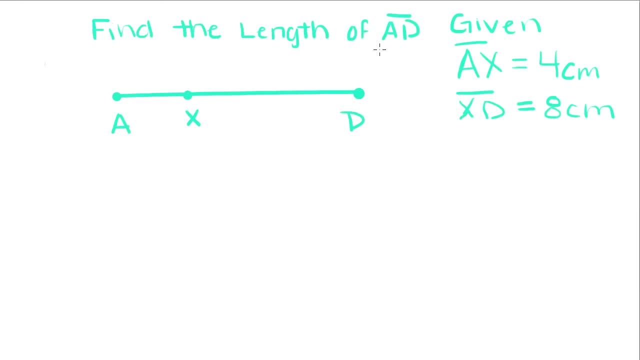 given that AX is equal to 4 centimeters and XD is equal to 8 centimeters, So we're just going to label this right here: 4 and 8.. And since this is what we're trying to find, we can add AX plus XD to find out what AD equals. 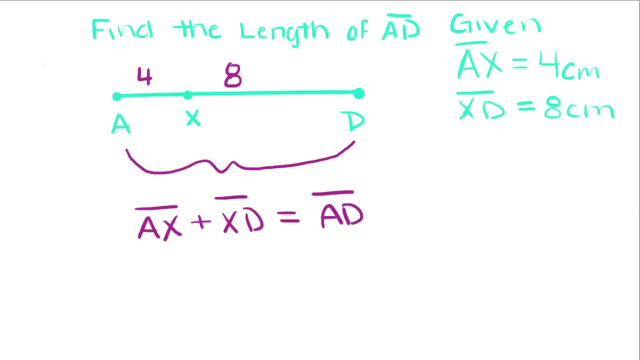 And this is called the addition property of segments And it allows us to take one part of the segment right here and add it to the other part of the segment to find the whole measurement of the whole segment. So all we do is we, since we know AX is 4 centimeters. 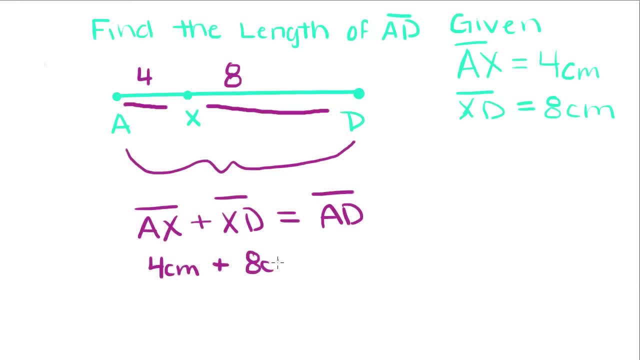 plus XD, which is 8 centimeters. we just add those together and you get 12 centimeters. Therefore, AD- the length of AD- is equal to 12 centimeters. Now, the only reason we can do this is because X lies in between AD. 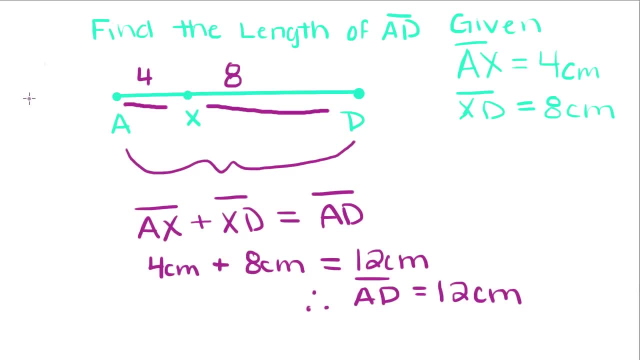 If X say X was over here somewhere And this was X, And we wanted to find the length of AD, We couldn't. we couldn't do anything with X. It's only because X is between A and D that we can add AX plus XD. 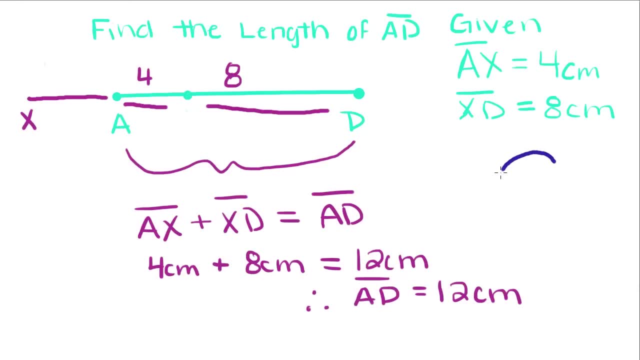 And this makes sense if you think about it, Because if you had a pizza and you had this much of a pizza, say, this is one-fourth of a pizza, and that's how much was eaten If the rest of it was also eaten. 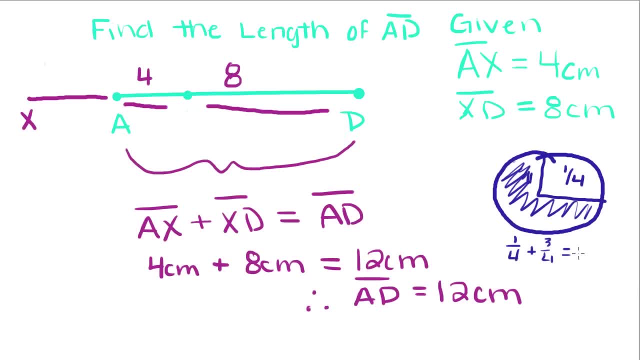 one-fourth plus three-fourths gives you the whole pizza. It's kind of like these are fractions of a line segment, So that to get the whole number you add each part together. Okay, So using those two definitions we just learned, 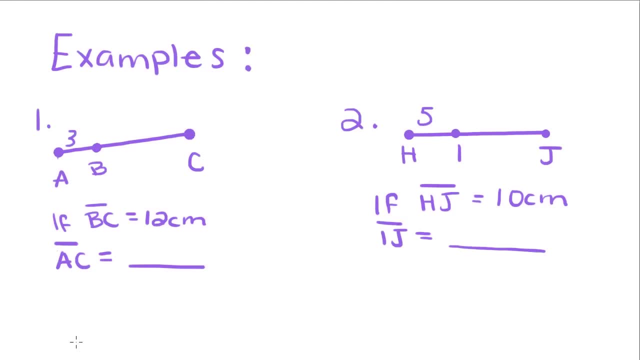 we're going to do some examples. Okay, So we already know that the length of AB is equal to three. That's already given to us right here. So they say: if BC is equal to 12 centimeters, how long is AC? 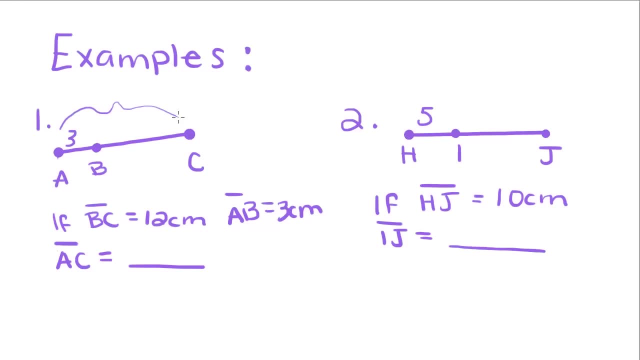 So since AC is the whole segment, we're going to take each part of the segments and add them together to find the whole length. So 12 centimeters plus 3 centimeters is equal to 15 centimeters. Therefore, AC equals 15 centimeters. 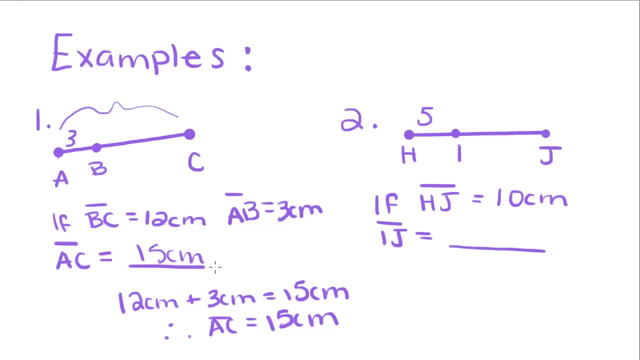 Alright. So on the second one, this one's a little different. They tell us what the whole length is. If HJ, which is the entire line segment, is equal to 10 centimeters, what is this part equal to? So, using the same idea, 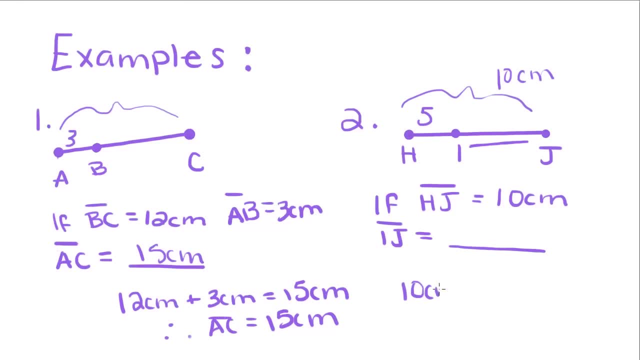 we're going to take the whole length minus part of the length to find out what the other part of the segment equals. And IJ equals 5 centimeters. Okay, For our last example, we're going to put the two things we learned together.